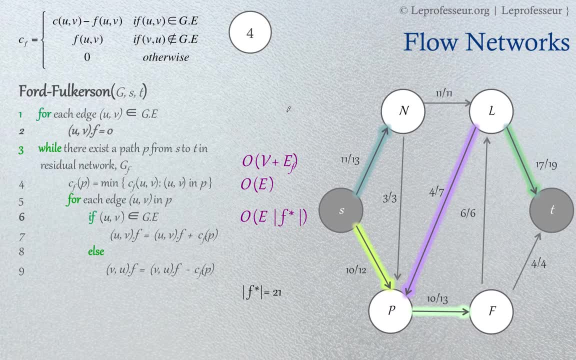 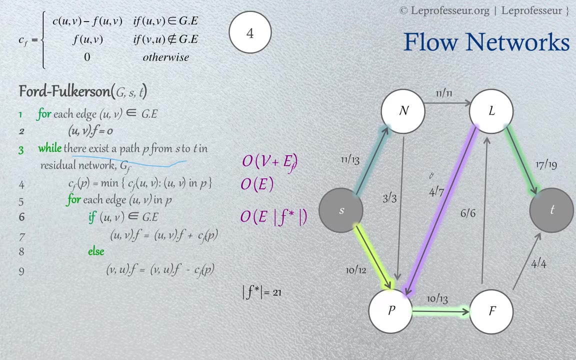 know that the Ford Phil Gerson's method- we call it a method, basically. so what it does, that it it finds a path. okay, it finds a path from source to destination in in our flow graph, in residual flow graph to be precisely, and the complexity was in the order of V plus E and the final complexity asymptotic value to: 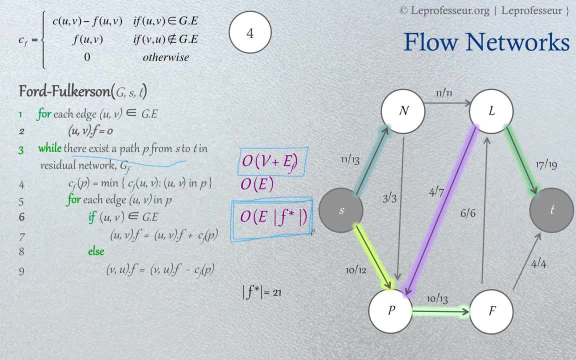 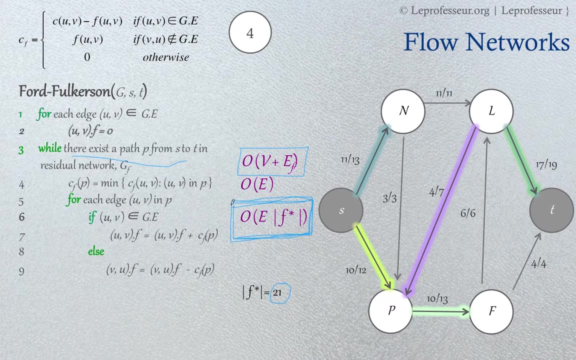 find the maximum flow value is in the order of edges multiplied by whatever is the maximum flow value in that order. so it's sort of: is there any way we can? we can have a bound on the complexity or we can reduce the complexity value because see, for example, if F is maximum flow value. 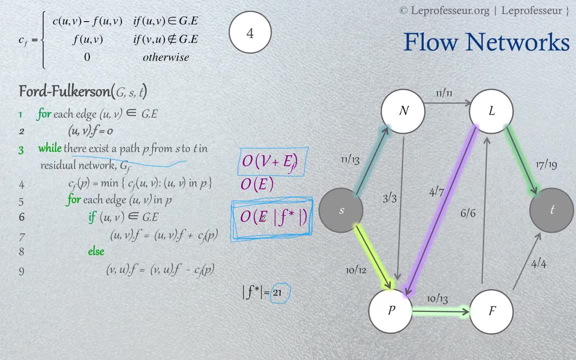 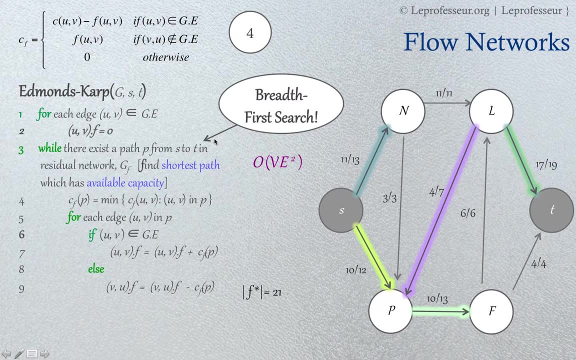 is a million and think about it, will have to do million operations. okay, now admins and carp these scientists. they came up with a novel idea that, instead of choosing a path, just any path at step number three in original force algorithm, what if we use breadth first, search and choose this shortest path? 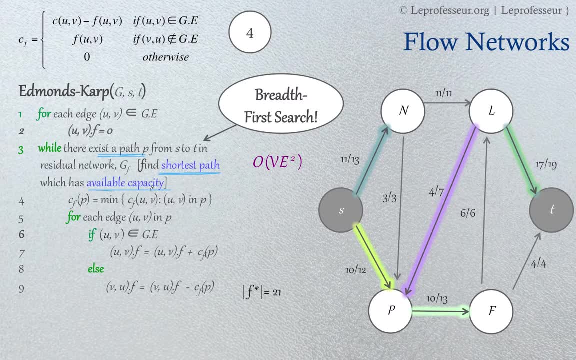 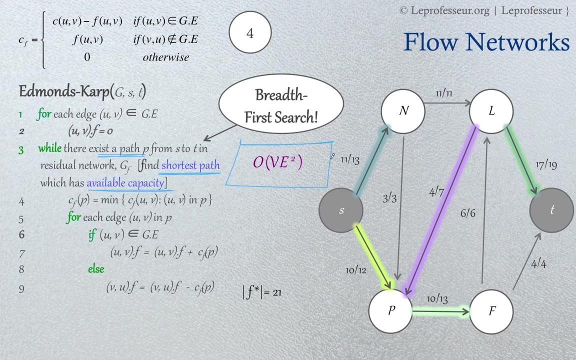 which has some available capacity left, so we can find the maximum flow value faster and in the order of V multiplied by E square, and that was a brilliant idea. so essential difference between these two algorithms is the way how the graph search is being implemented. you So, if you're going to use breadth-first search and you're going to select sort test path.